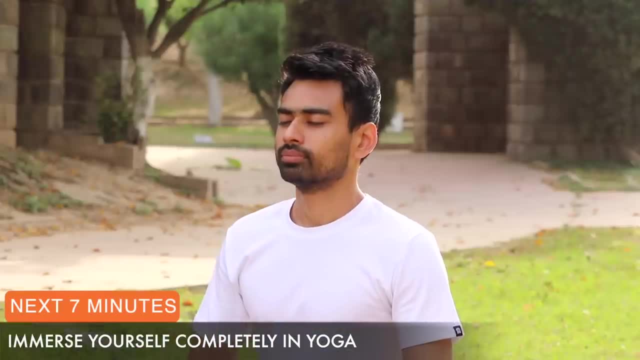 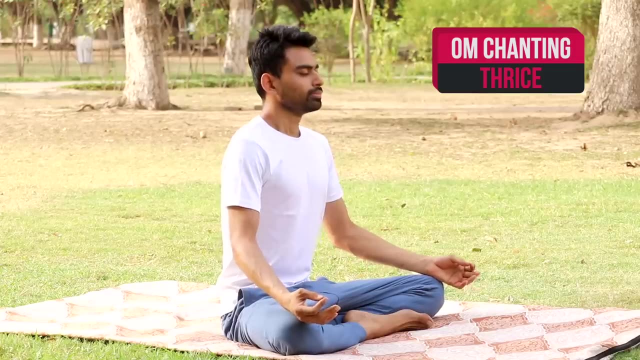 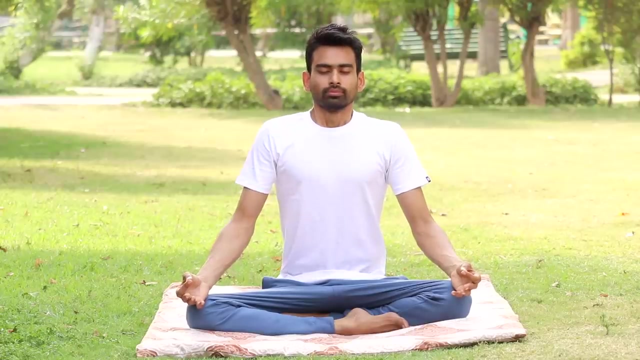 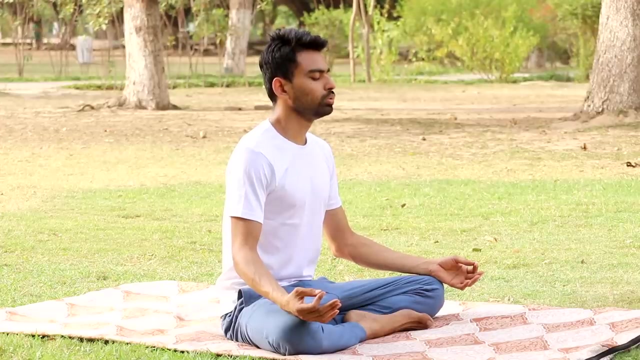 For the next 7 minutes, let's immerse ourselves completely in this divine practice. We will start with chanting OM three times: Spine, erect, neck, straight hands in Dhyan Mudra, close your eyes, Take a deep breath in and exhale out. chanting OM, OM is not a sound of any one particular religion. 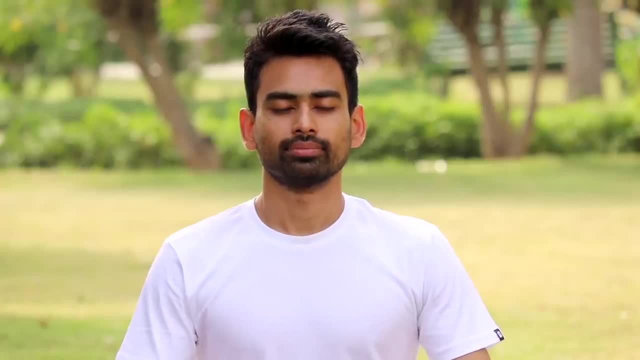 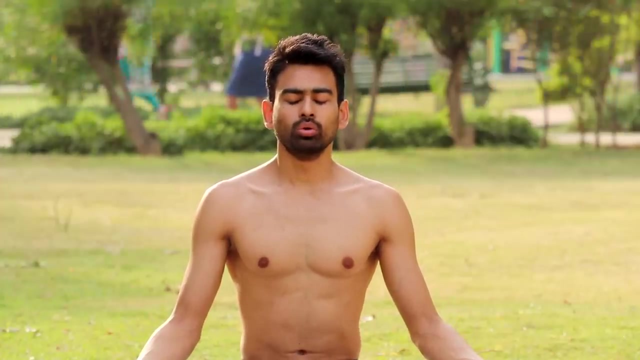 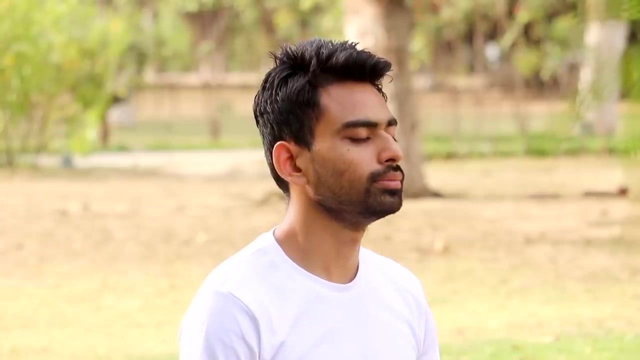 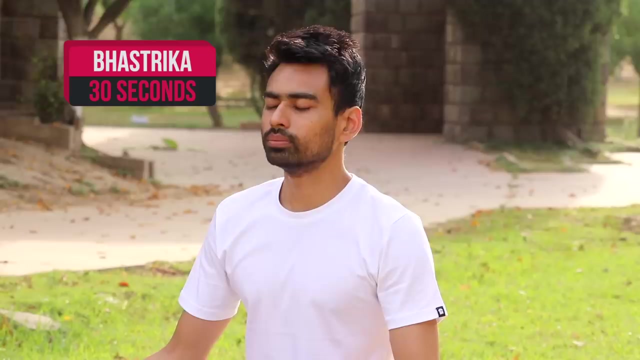 It is the sound of creation which encompasses all sounds within. OM is the sound of oneness. The vibrations of this sound harmonizes the body for a deep yoga session. Relax, keep your eyes closed. Now we will do. Bhastrika, also known as bellows: breath for 30 seconds, Alright, deeply, breathe in forcefully. 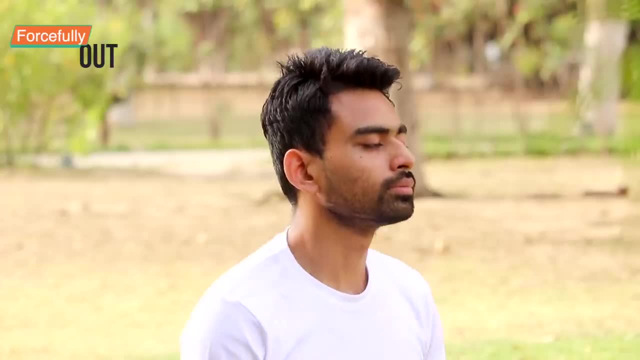 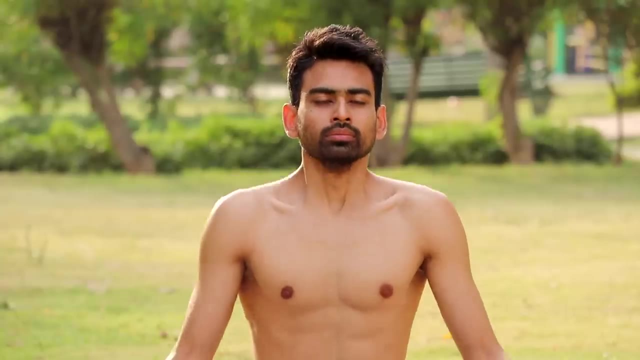 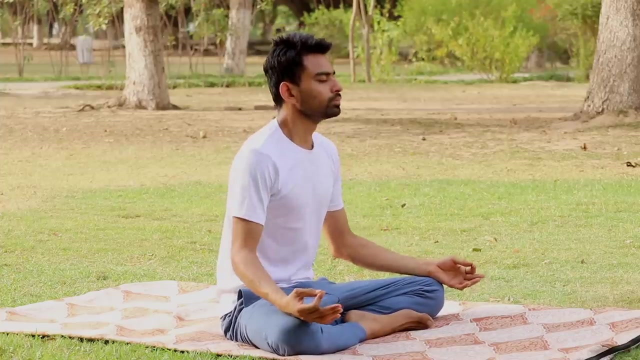 breathe out, in, out, in out. Maintain the same rhythm, breathing in and out through your nostrils. This is the yogic breath of fire which energizes the body almost instantly. Do it with undivided attention. Feel that with every inhalation, positive energy is entering your body. 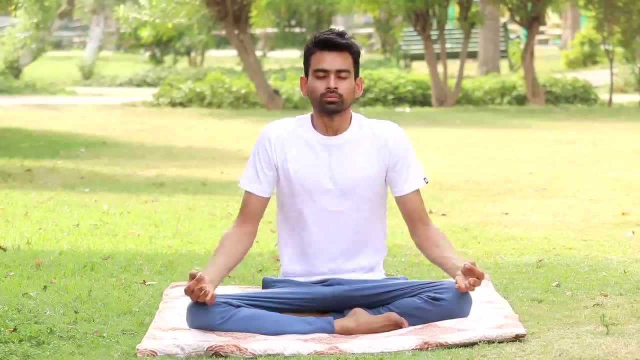 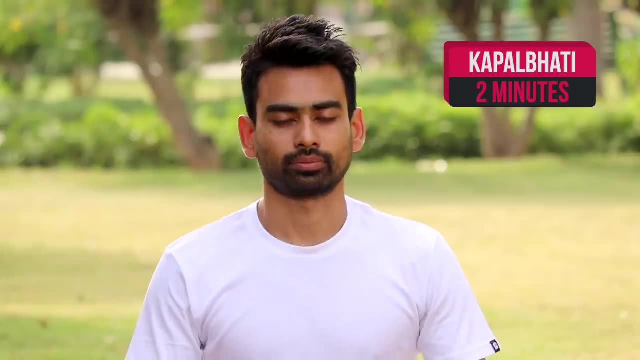 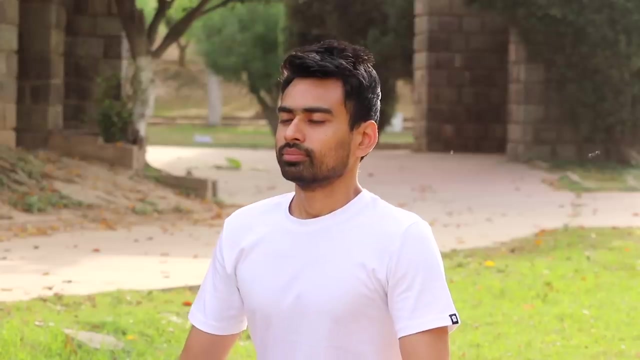 And with every exhalation the negativity is being pushed out. Relax, keep your eyes closed. Now, for the next two minutes, we will do Kapalbhaati, also called rapid exhalation. I will start with counting, and with every count you have to exhale out through your nostrils. 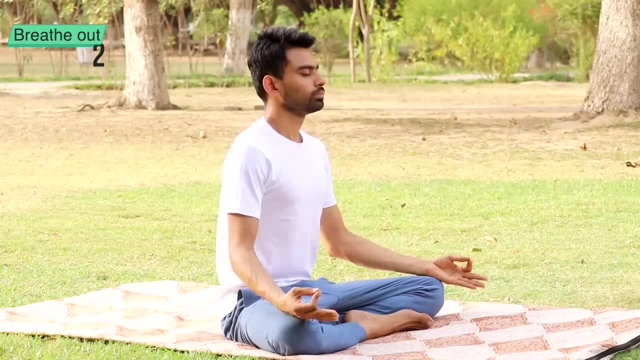 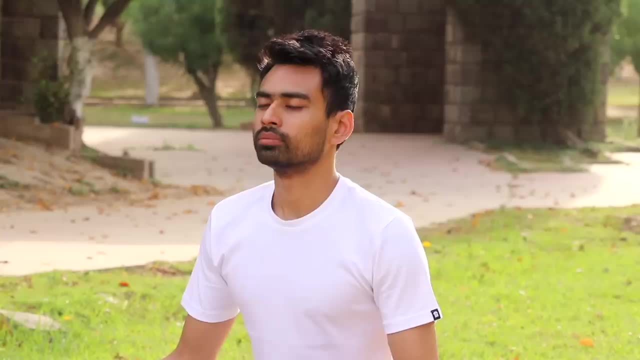 Take a deep breath in and 1,, 2,, 3,, 4,, 5,, 6,, 7.. Maintain the same rhythm. You can keep counting in your mind if you so wish. However, at no point over exert yourself. Keep a. 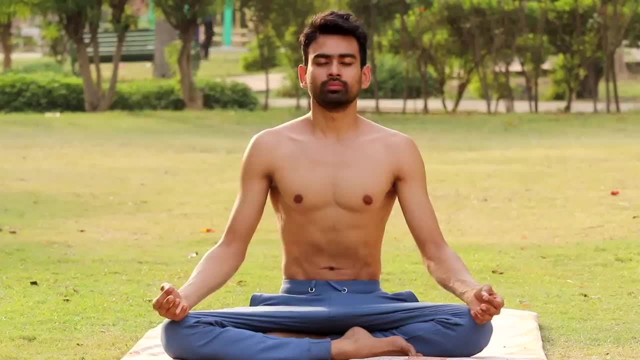 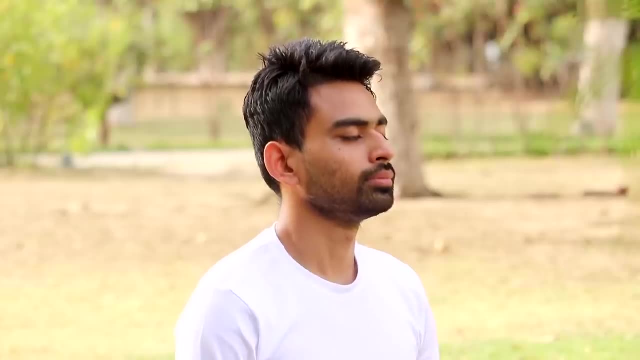 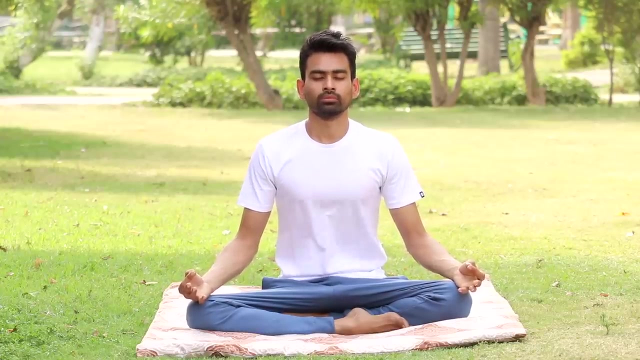 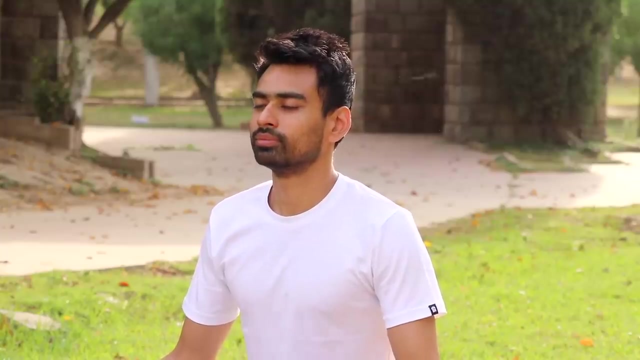 smile on your face, radiating positivity. Throughout this Kriya, keep your attention fixed on the abdominal area. It will enhance its effect many folds. This is where the Manipurka chakra is located. Feel that your abdomen is being massaged, The subtle channels are being opened up, The toxins are being pushed. 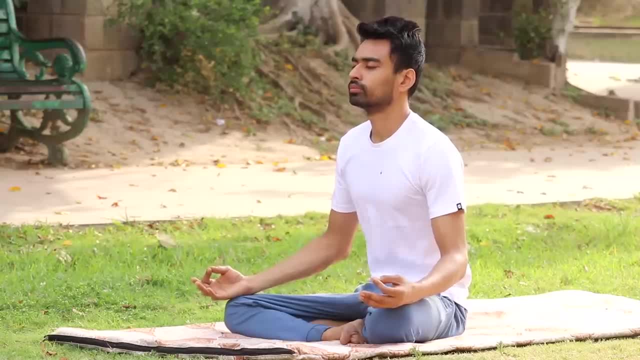 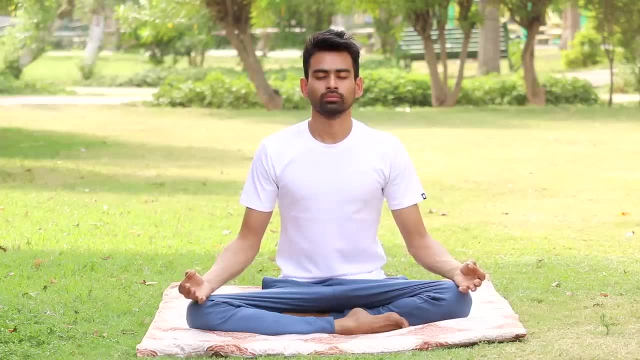 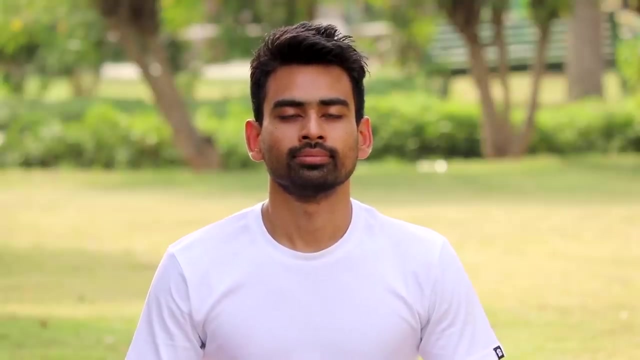 out. The internal factory is being cleansed. This is the yogic lung purification. Just keep breathing out. It so effectively circulates the blood in the entire body that in yogic scriptures, Kapalbhati has been equated to sprinting. Do it with complete involvement. 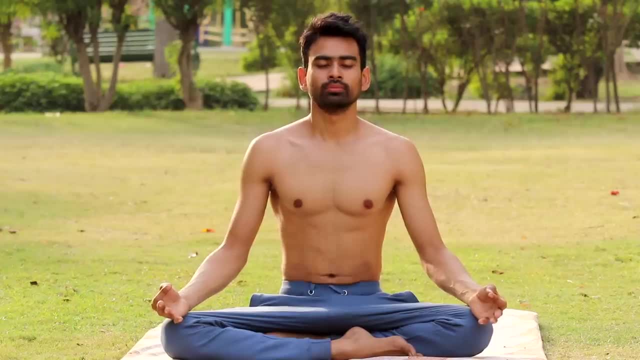 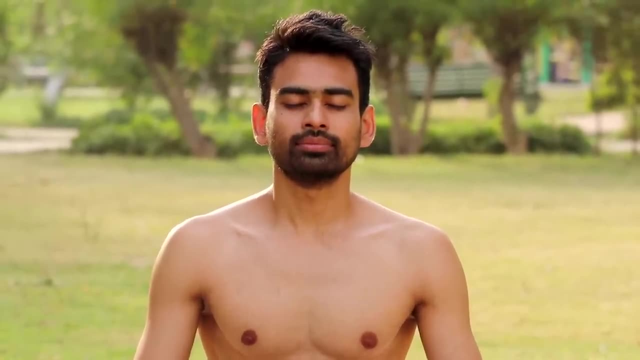 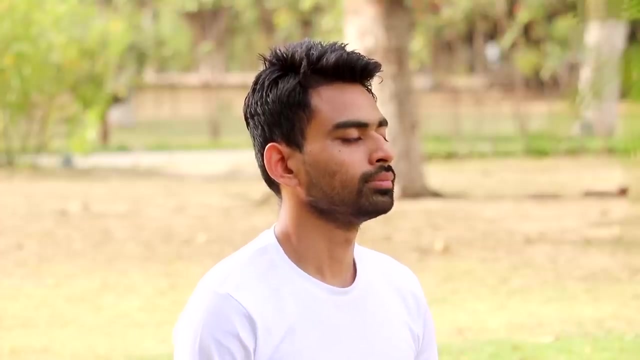 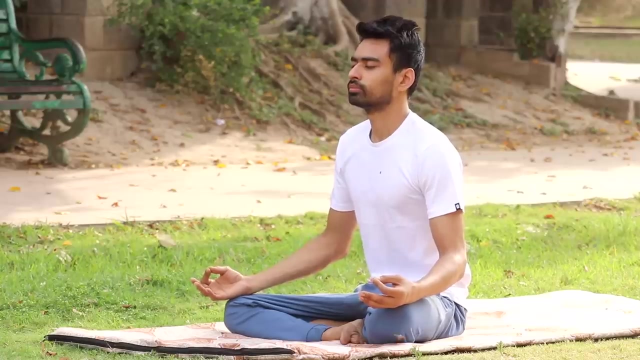 you Focus fixed on the abdominal area. Over 95% of the diseases originate from the stomach, which is why regular practice of Kapalbhati has such a profound effect on health. The 72,000 nadis, or the subtle channels of which we are made of, Kapalbhati has the power to. 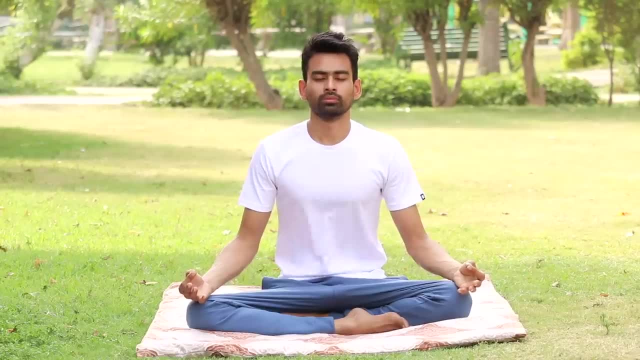 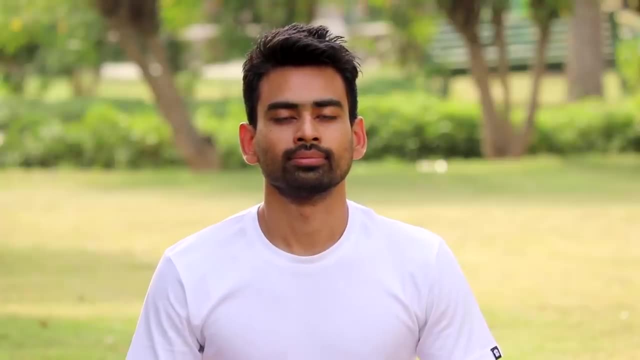 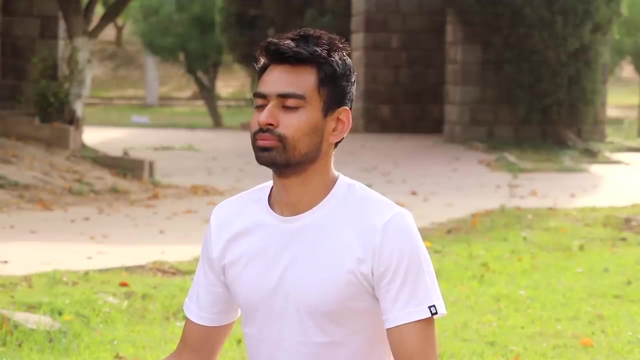 clear its pathways, Since Kapalbhati helps detoxify the complete mind-body system. when consistently practiced, the face shines, which is also why it is named so: Kapala, meaning the skull, and Bhati, meaning shining. Simple, yet an advanced practice for overall well-being. 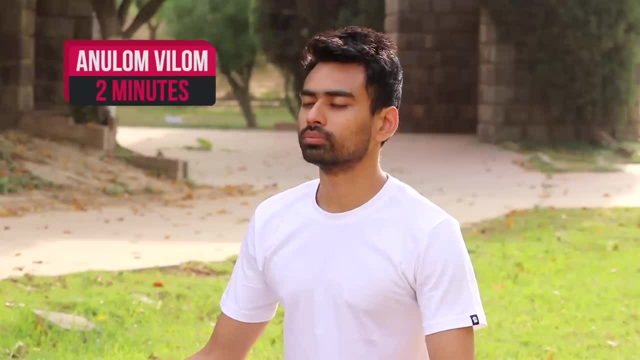 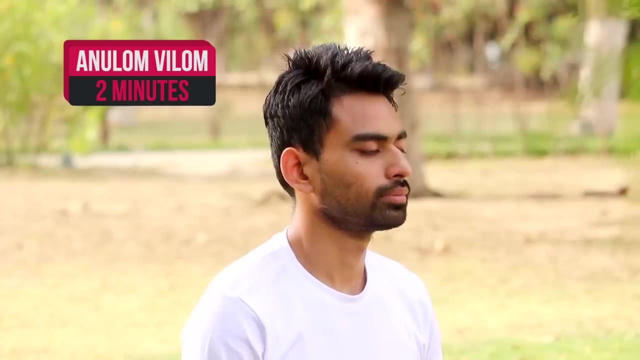 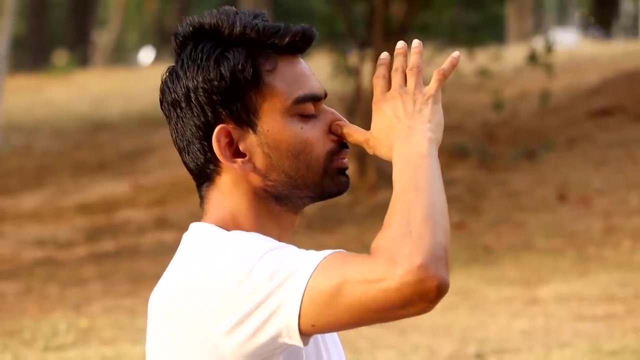 Relax Now. for the next two minutes we will do alternate nostril breathing, commonly known as Anulom Vilom Pranayam. such a calming exercise: Using the right thumb, block the right nostril, Inhale through the left nostril for 4 seconds. 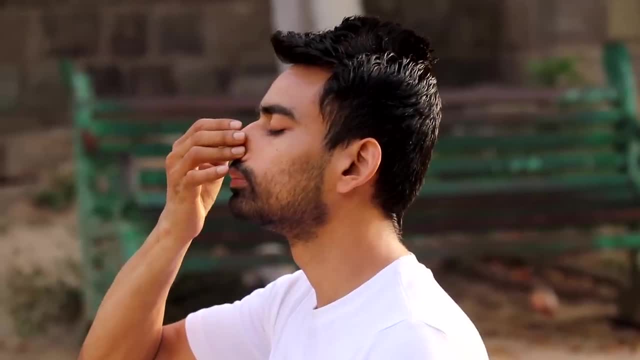 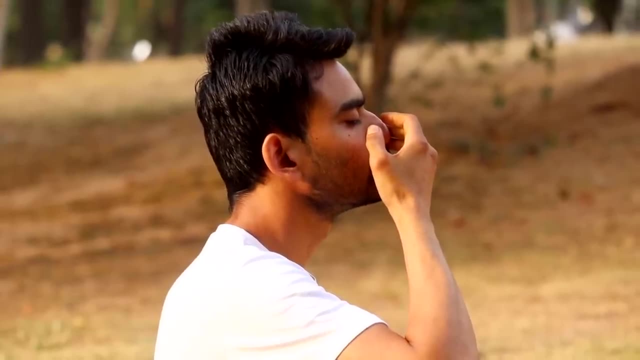 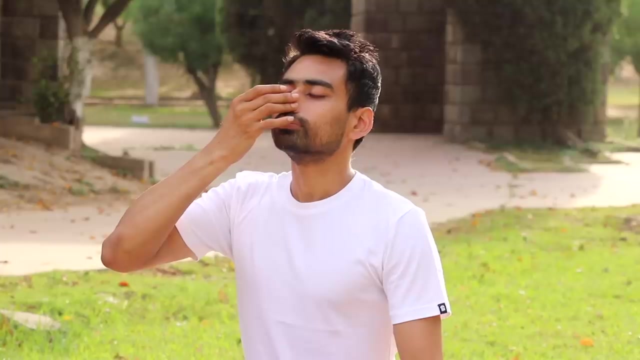 Hold there for 4 seconds. Then, placing the middle two fingers, close the left nostril and exhale through the right nostril for 4 seconds In the same position. inhale through the right nostril for 4 seconds. Hold for 4 seconds. 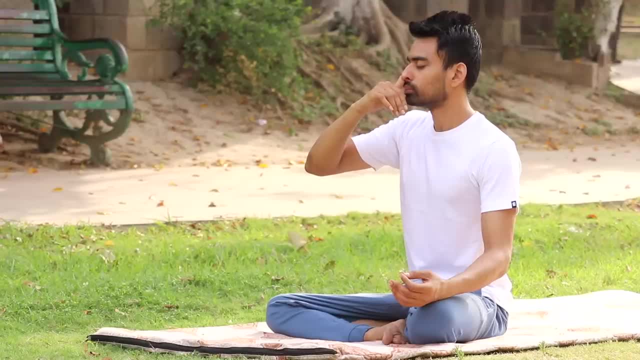 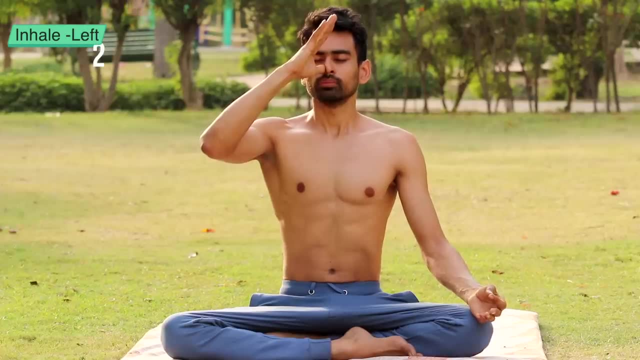 Place the right thumb to block the right nostril and exhale through the left nostril for 4 seconds. Repeat: Inhale 2, 3, 4.. Hold 2, 3, 4.. Exhale 2, 3, 4.. 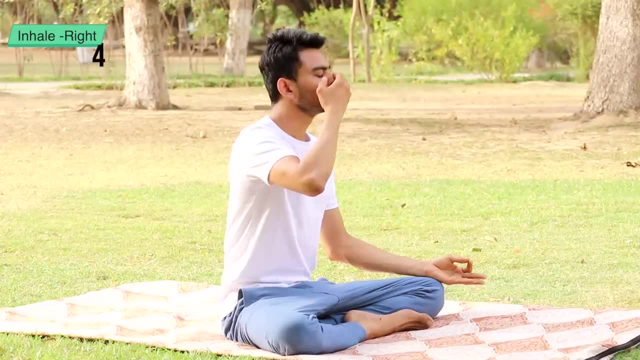 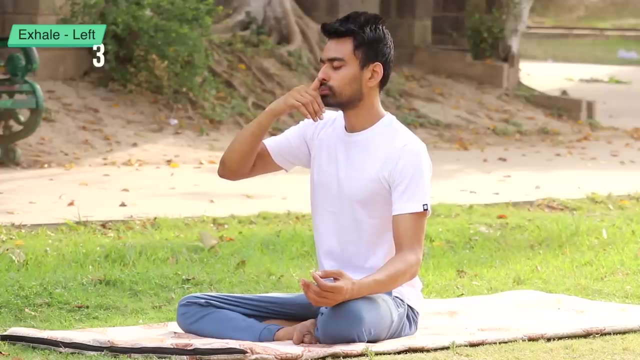 Inhale 2, 3, 4. Hold 2.. Exhale 2, 3, 4.. Inhale 2, 3, 4.. Hold 2, 3, 4.. 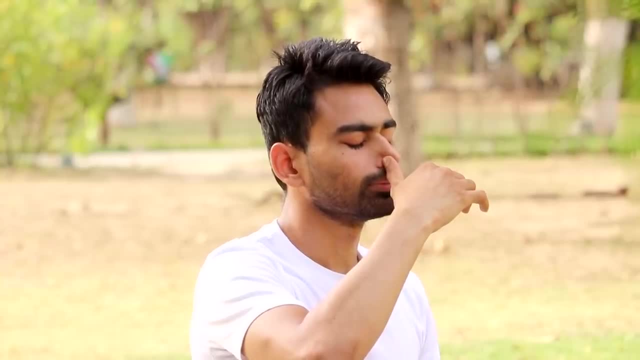 Exhale 2,, 3,, 4.. Maintain the same rhythm, keeping a mild focus in between your eyebrows. Maintain the same rhythm, keeping a mild focus in between your eyebrows. This is an advanced form of alternate nostril breathing. 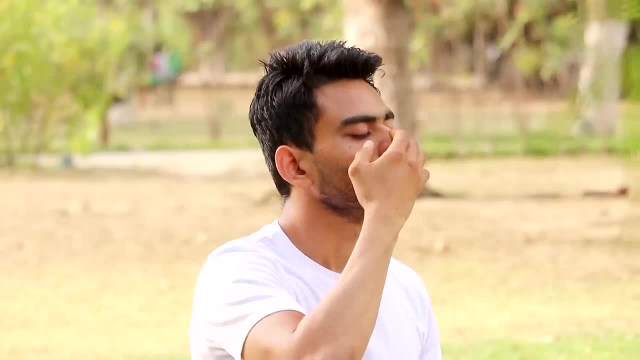 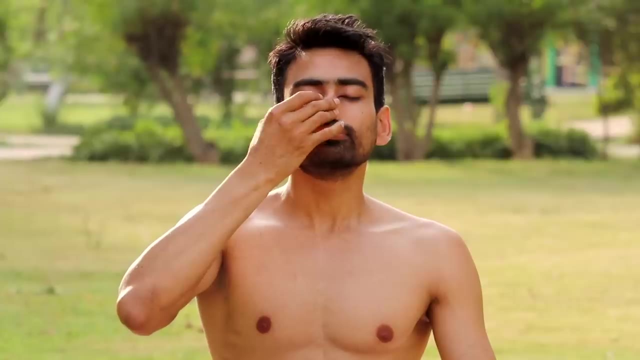 This is an advanced form of alternate nostril breathing. Long inhalation oxygenates the blood, breath retention strengthens the nervous system and long exhalations eliminate carbon dioxide. And long exhalations eliminate carbon dioxide, Also called the Nadi Shodhan Pranayama. 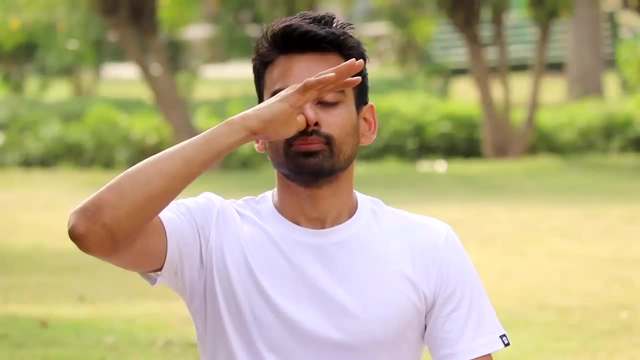 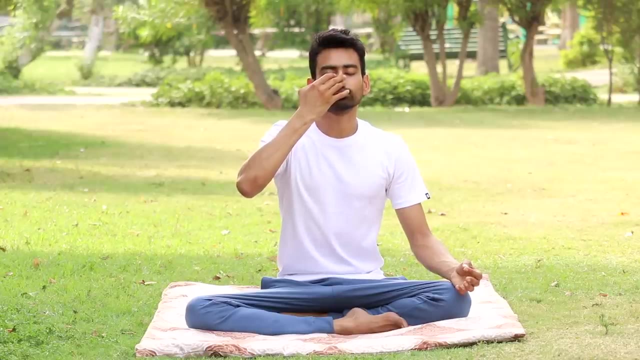 as it purifies the two most important nadis, Ida and Pingala. Stress, anxiety, depression, you name it. Anulom Vilom has the capacity to destroy it from its root. Anulom Vilom has the capacity to destroy it from its root. 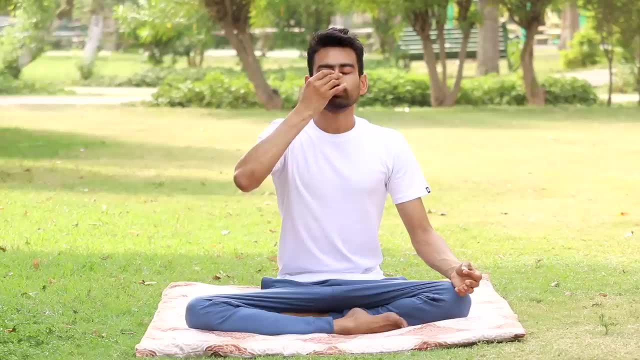 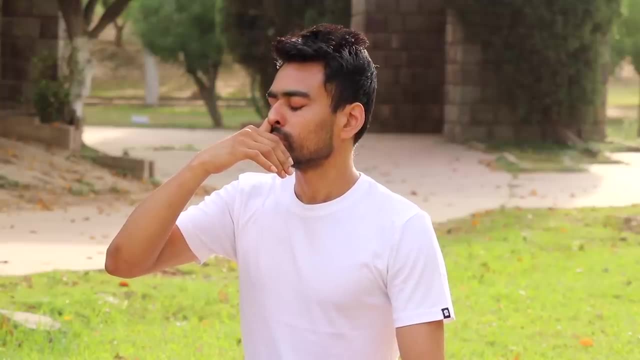 Do it with total involvement. Feel the system getting revitalized. Feel the system getting revitalized. Feel the impurities are being brought out. Feel the impurities are being brought out. Feel the impurities are being brought out. Anulom Vilom is getting lighter. 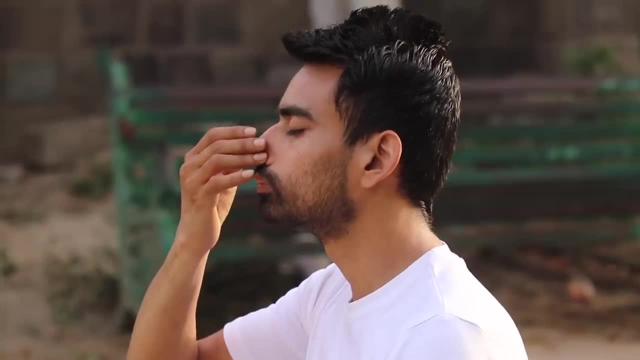 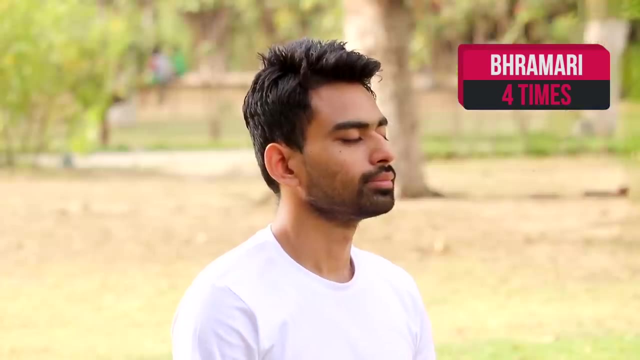 Such deep cleansing. Anulom Vilom, the ultimate therapy. Anulom Vilom, the ultimate therapy, The last breathing exercise of this session. The last breathing exercise of this session is the Brahmari or the B-Breath Thumbs, closing the ears. 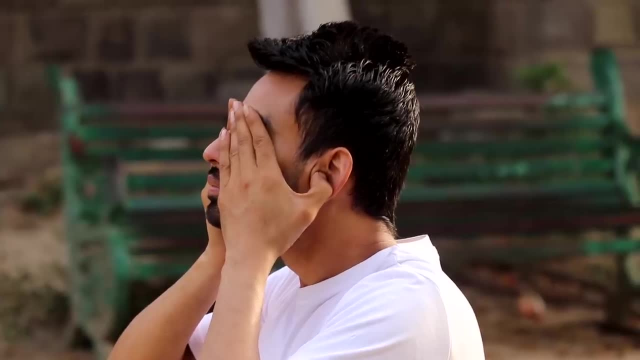 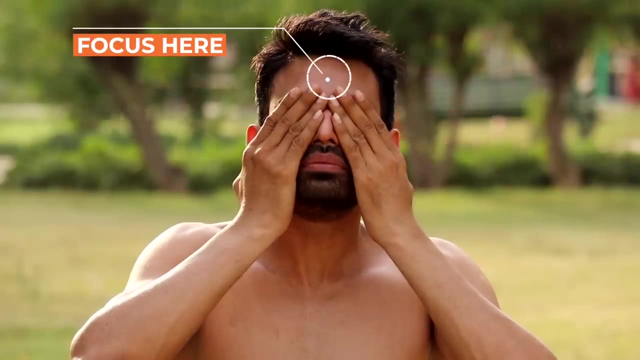 Index fingers just above your eyebrows and the rest of your fingers softly placed over your eyes. Touch the tip of your tongue to the palate. Touch the tip of your tongue to the palate. Focus in between your eyebrows. Focus in between your eyebrows. Inhale deeply through your nostril for 4 seconds. 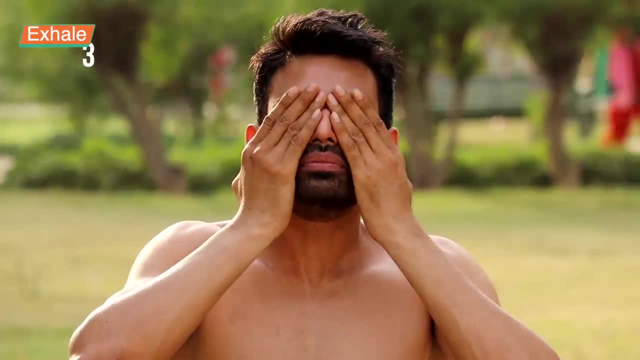 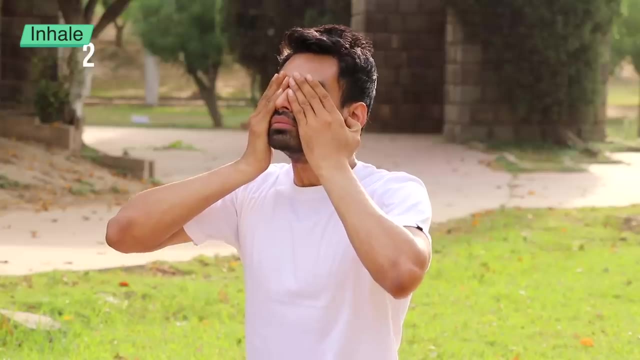 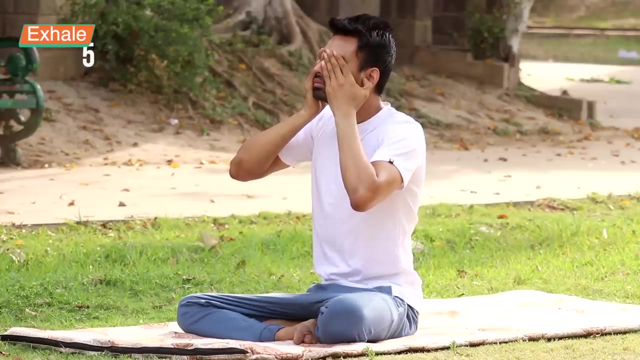 and exhale making a humming sound of and exhale making a humming sound of OM for 8 seconds. OM for 8 seconds. Inhale: 2,3,4, 2,3,4, 2,3,4, 2,3,4. 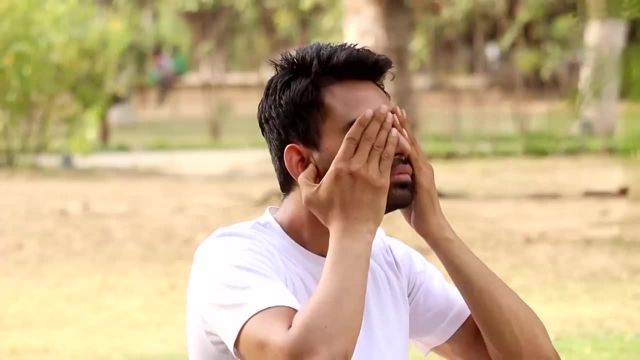 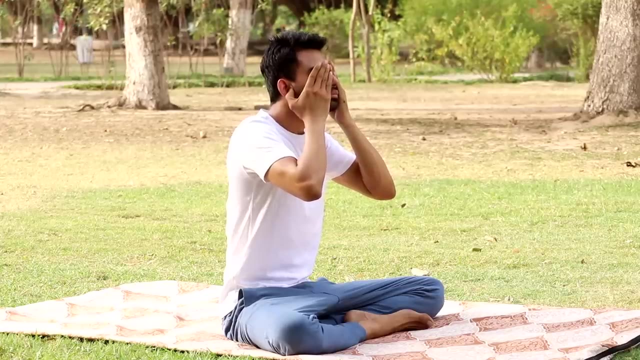 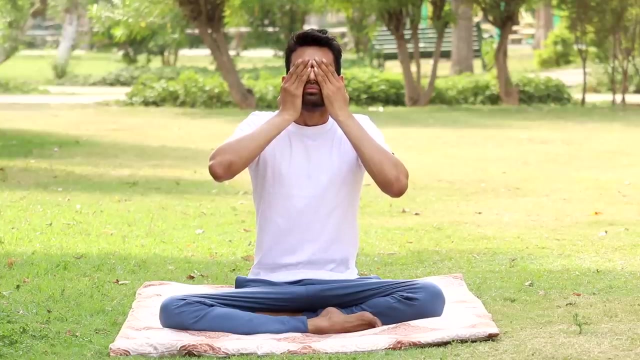 2,3,4. The vibrations of this divine sound balances the body and mind, cleansing the aura OM. Visualize that your body is radiating positive rays in the form of humming sound of the bee, Activating the pineal and pituitary glands. 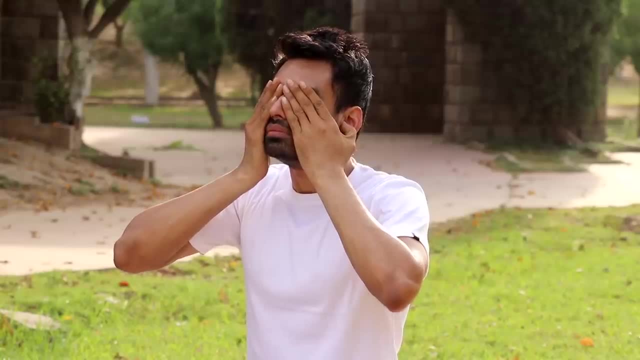 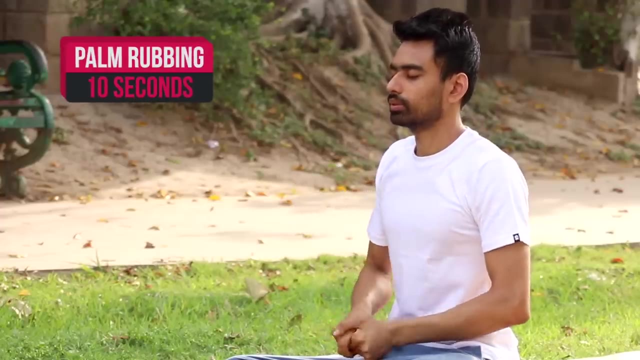 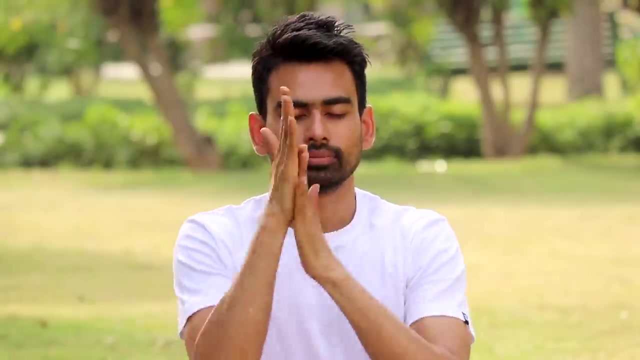 OM. It is an elixir for all brain disorders. Now, before opening the eyes, bring your palms together in front of your face and rub them with vigor for about 10 seconds. This will stimulate the acupressure points, allowing better flow of prana Place, the 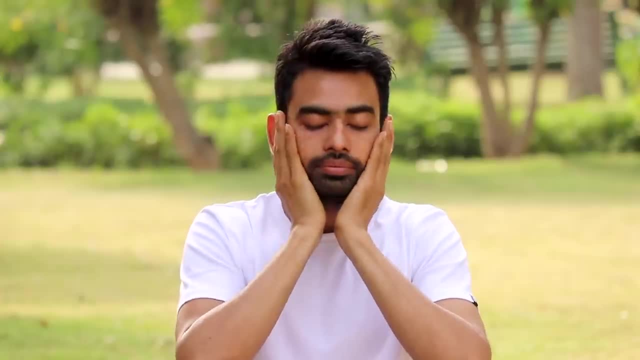 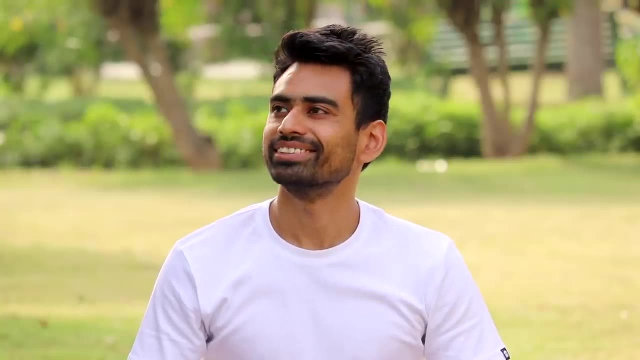 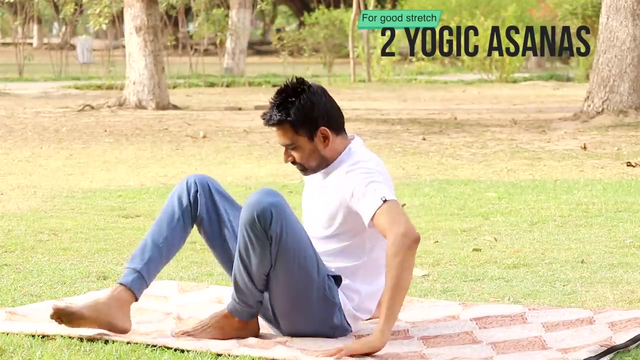 palms softly over the eyes. Feel the warmth. It heals the eyes. Now slowly open your eyes. This is the moment of tranquility, calm, harmony. But before we wrap up, lie down to quickly do 2 yogic asanas that will provide a good stretch. 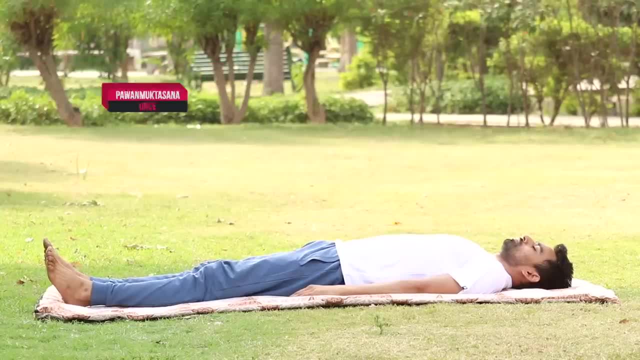 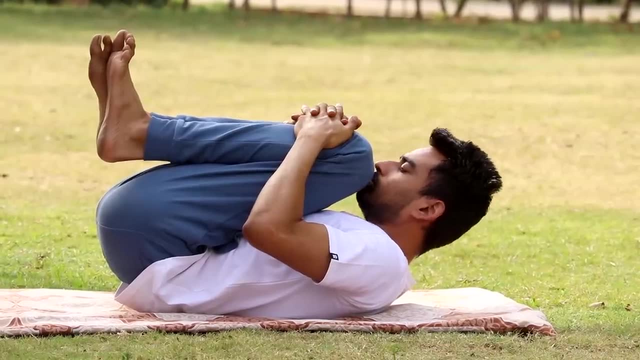 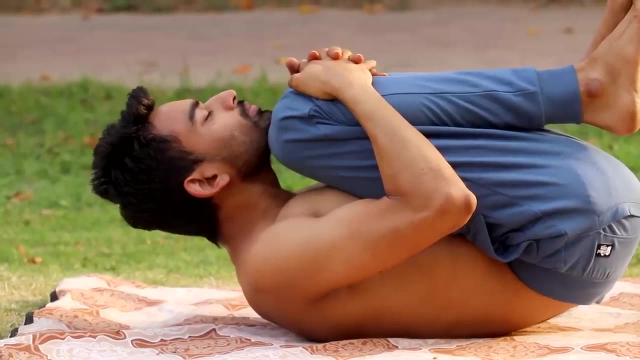 First is the Pavanmuktasana. Breathe in and, as you exhale, bend your knees, interlock your fingers, lift your head to first touch your nose and then chin, Hold there for 10 seconds, Enhancing the blood circulation in the pelvic. 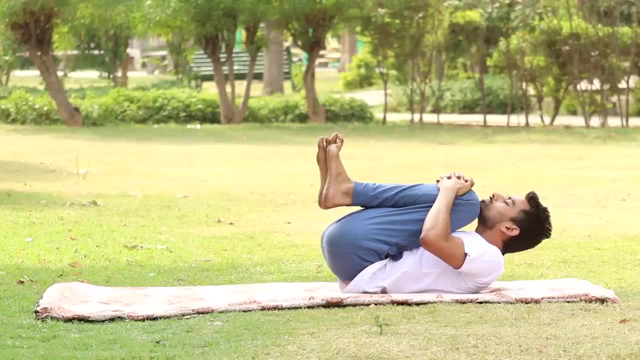 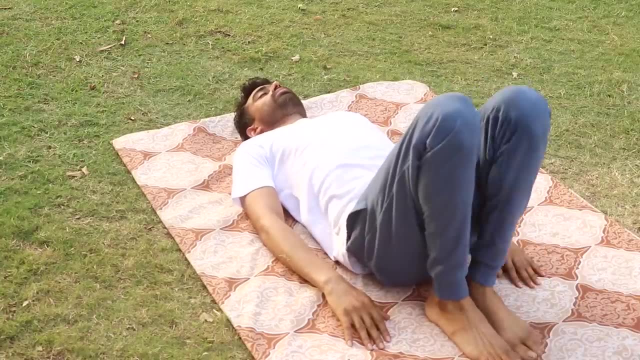 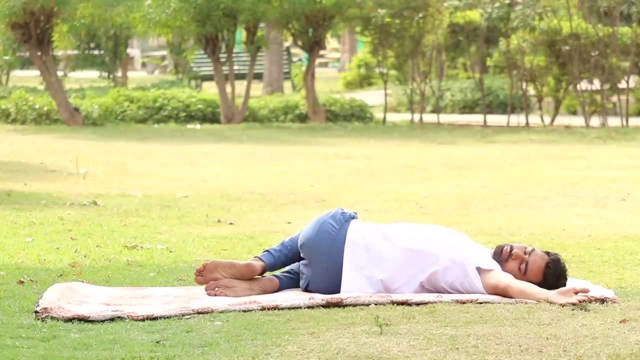 region. this relieves excess wind in the system. Relax. Now we will do Markatasana. Bend your knees and keep your feet close to hips. Spread your arms wide. Now turn your knees together to right while neck to left. Hold there for 10 seconds. 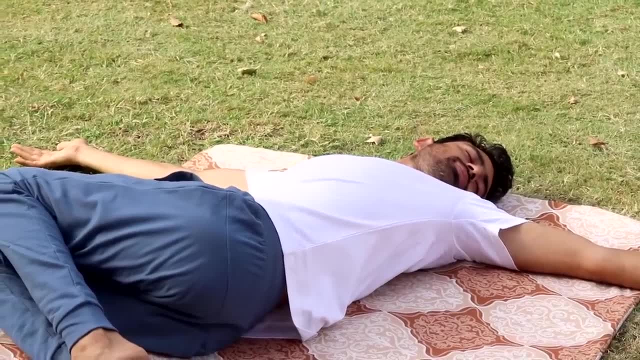 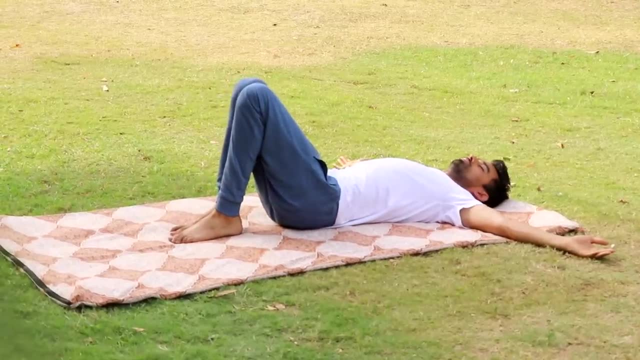 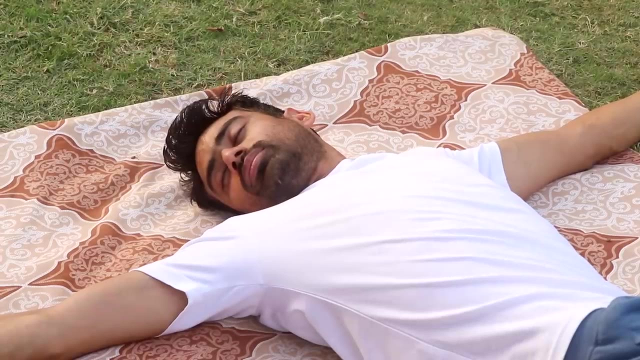 Breathe normally. Feel your back, neck and shoulder muscles getting stretched. Now move your knees to the left while the neck to the right Again. hold for 10 seconds. Markatasana is probably the best remedial posture for back pain. 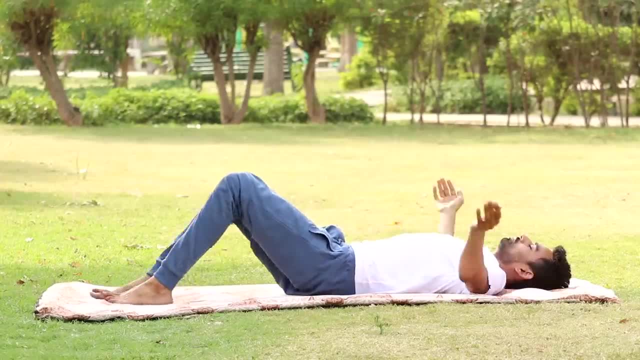 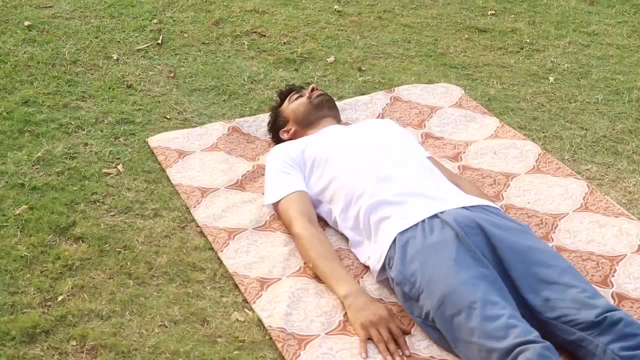 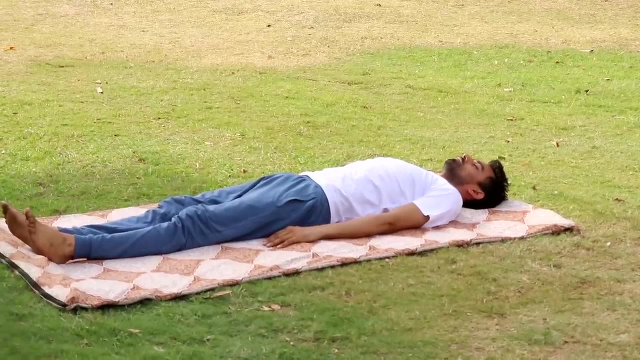 Relax. Keep lying down on the mat in Shavasana for about 30 seconds. It is the yogic cool down. Close your eyes and feel the sensations in the body. Be aware of every moment. Your mind and body is thanking you for having. 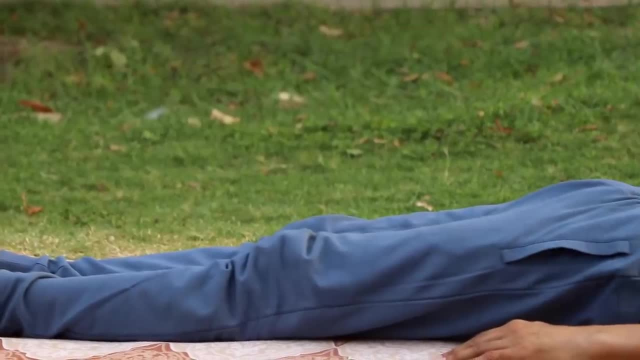 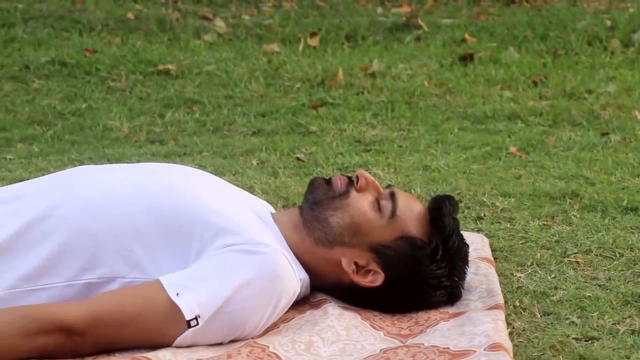 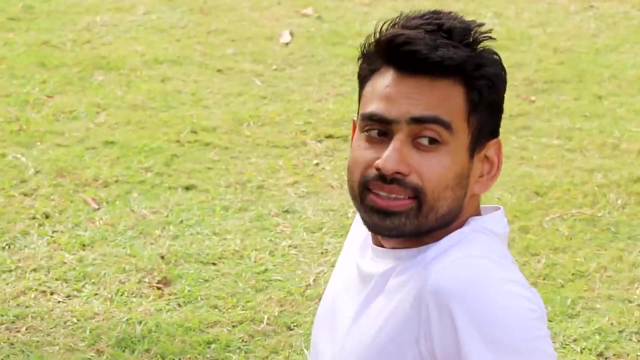 completed this yoga session. Every organ, every cell in your body is feeling delighted to have been taken care of. Be proud of yourself. You have done it. You will bow down to the divine within you. I will see you tomorrow, Namaste.